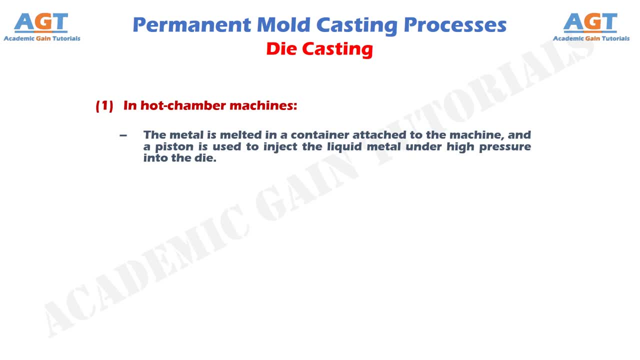 is used to inject the liquid metal under high pressure into the die. Production rates up to 500 parts per hour are not uncommon. Hot chamber die casting imposes a special hardship on the injection system because most of it is submerged into the molten metal. Hence the applications. 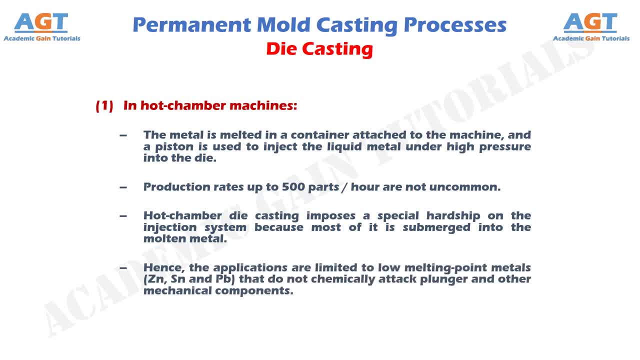 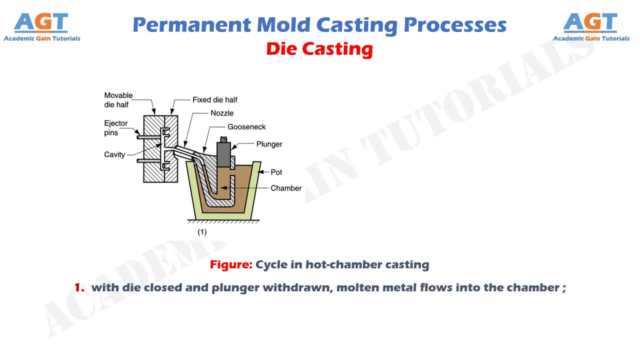 are limited to low melting point metals- zinc, tin and lead- that do not chemically attack plunger and other mechanical components. The figure 1, shows the first step in hot chamber die casting, where a with die closed and plunger withdrawn, molten metal flows into the chamber. 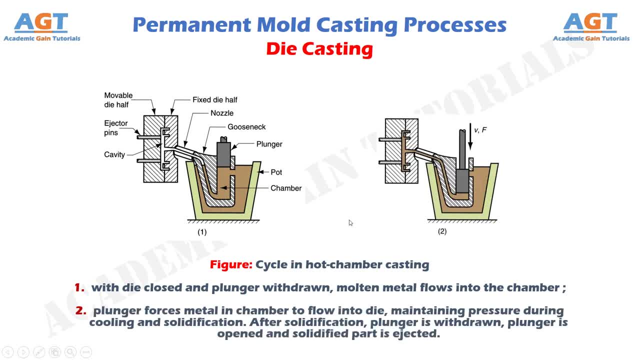 The figure 2, shows the second step in hot chamber die casting, where the plunger forces metal in chamber to flow into die maintaining pressure during cooling and solidification. After solidification: plunger is withdrawn, plunger is opened and solidified part is ejected. 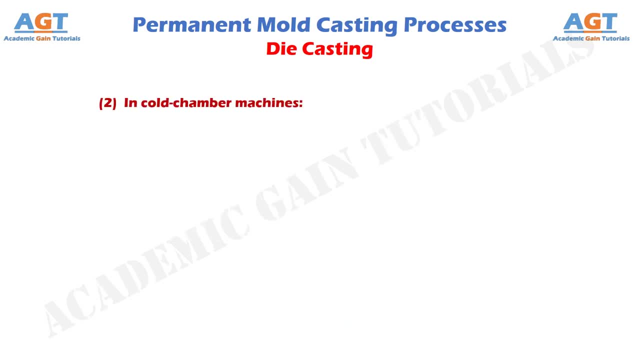 On the other hand, in cold chamber die casting machines, the molten metal is poured into an unheated chamber from an external melting container and a piston is used to inject the metal under high pressure into the die cavity at about 14 to 140 MPa Compared to hot chamber. 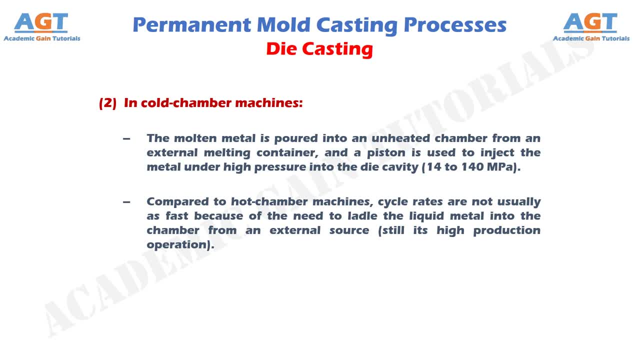 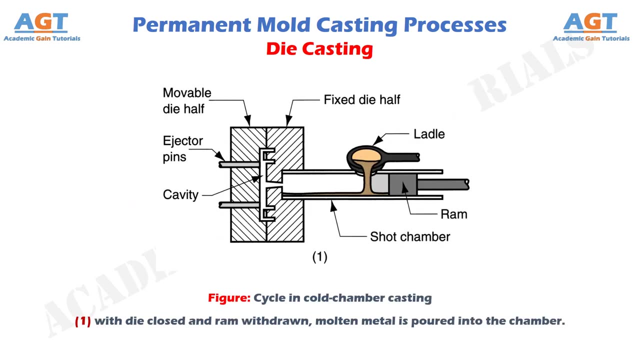 machines cycle rates are not usually as fast because of the need to let the metal flow into the die cavity at about 40 MPa. Conclusion: The figure 2, shows the first step in cold chamber die casting, where a with die closed and ramp withdrawn, molten metal is poured into the chamber. 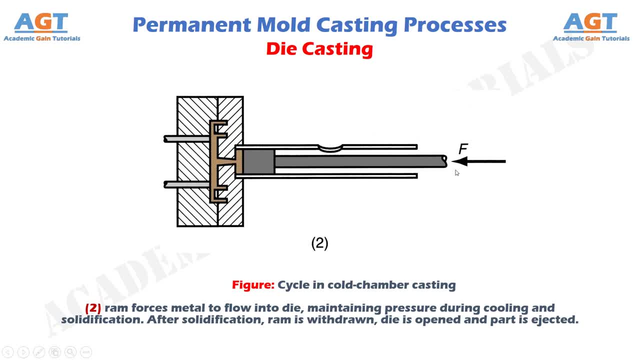 The figure 2, shows the second step in cold chamber: die casting, where the ramp forces metal to flow into die, maintaining pressure during cooling and solidification. cooling and solidification: After solidification, ram is withdrawn, die is opened and part is. 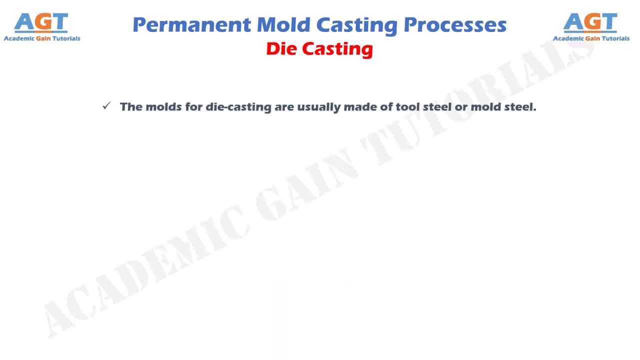 ejected. The molds for die casting are usually made of tool steel or mold steel. Tungsten and molybdenum with good refractory qualities are also used. Ejector pins are required to remove the part from the die when it opens. Lubricants must be sprayed into the cavity to prevent.